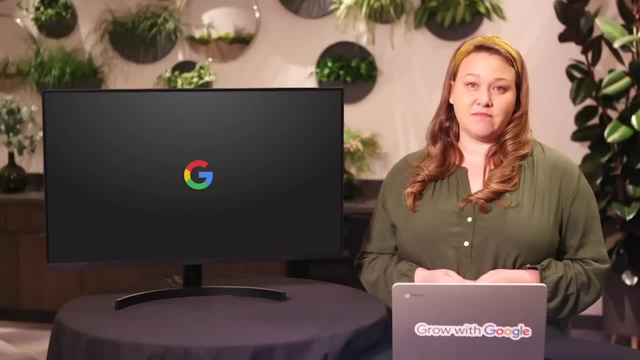 was very different. As the technology was changing, it was becoming increasingly difficult to decide what to look for During World War I. the sheer number of men and women needed for the war effort made it impossible to choose specific people for specific tasks. Aviation design had to consider. 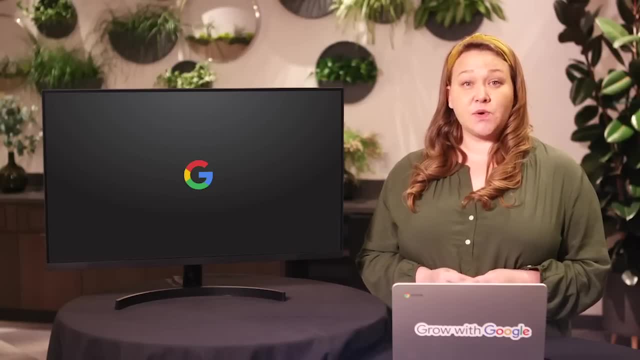 human factors. In this case, human factors were the pilot's varying skill levels. If we were robots, some computer genius could just program us to be expert fliers, But we're only human and not everyone can fly, So we had to learn how to fly to the highest places in the world, including the 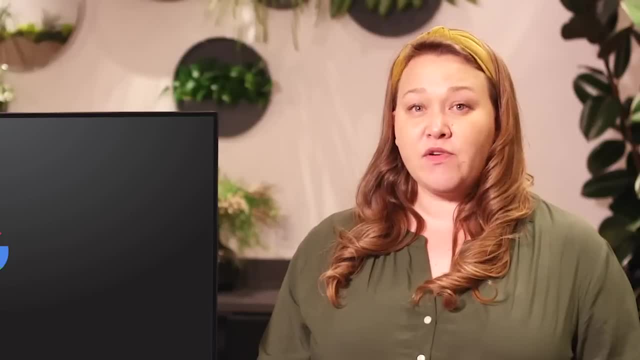 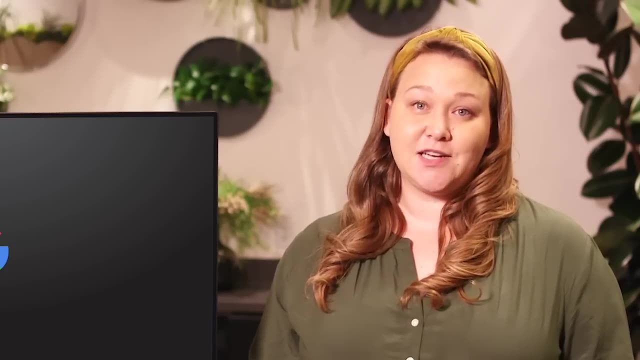 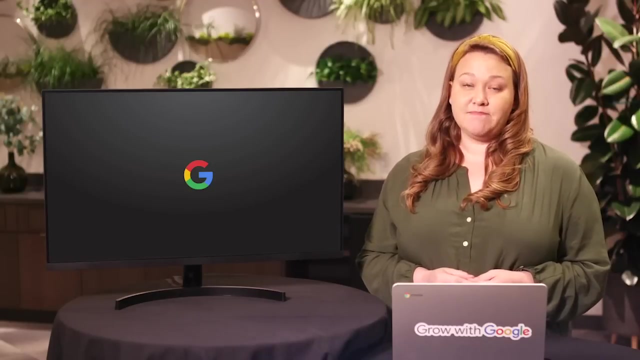 flying a warplane was an ace pilot. To account for this human factor, we had to adapt the plane to the pilot, And by World War II we finally had the tech to do it. So what are some of the human factors that inform design? Here's a few of the most common ones: Impatience, limited memory. 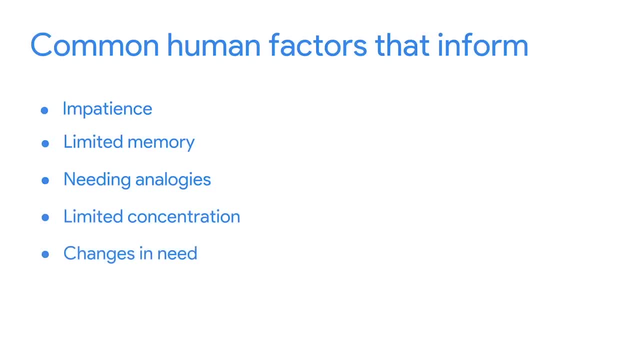 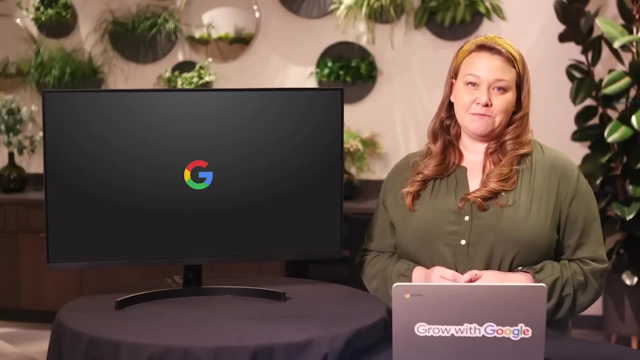 needing analogies, limited concentration, changes in need. needing motivation, prejudices, fears, making errors and misjudgment. For an example of design that considers these factors, all you need to do is check your email, The business email shorthand. TLDR has really caught. 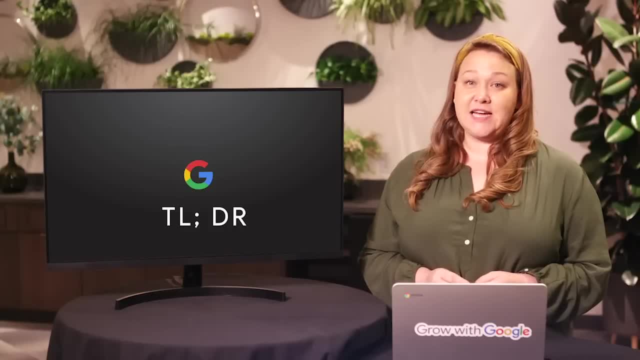 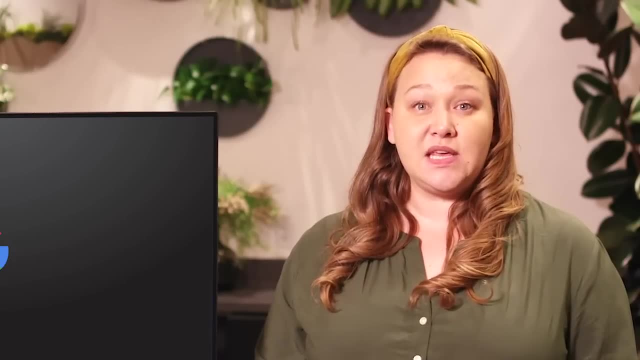 on in the last couple years. It's an acronym you might find at the start of a very long email. A TLDR is a short, succinct summary that only gives you the email highlights you really need to know, without any excess content. So what does TLDR mean? It's a short, succinct summary. 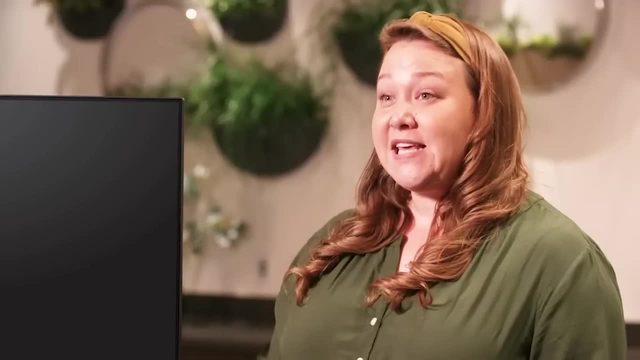 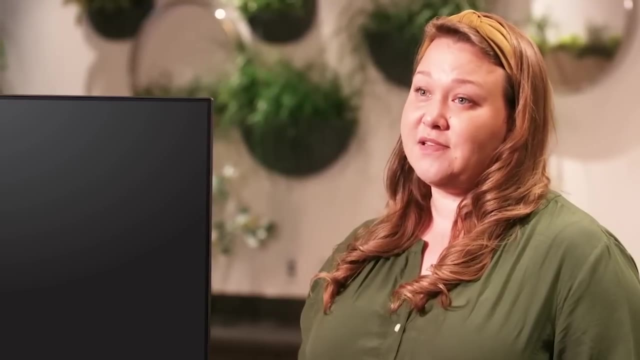 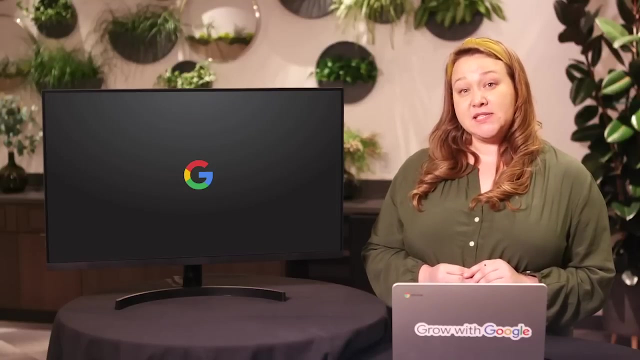 that says what does TLDR stand for? Too long didn't read The email writer. factors in the human tendencies of impatience, limited concentration, need for motivation and limited memory. Not bad for four little letters. Here are psychological concepts that can help you design. 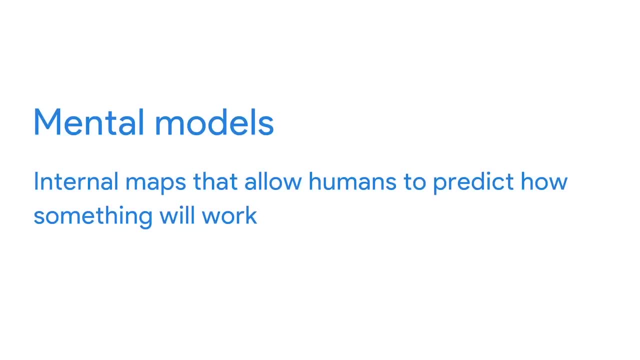 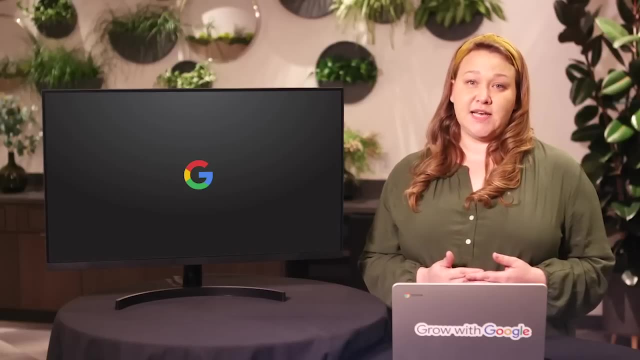 with the human factor in mind. Mental models are internal maps that allow humans to predict how something will work. When you face a door, your mental model tells you that the door can be opened. Once the door is opened, you'll be able to leave the room. The process of opening the door. 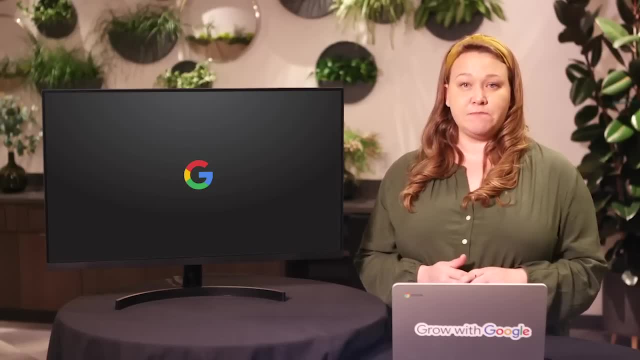 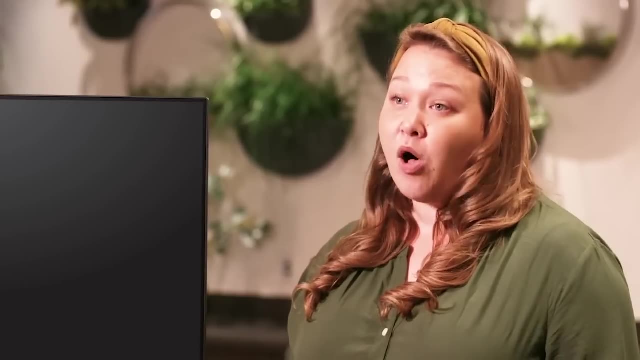 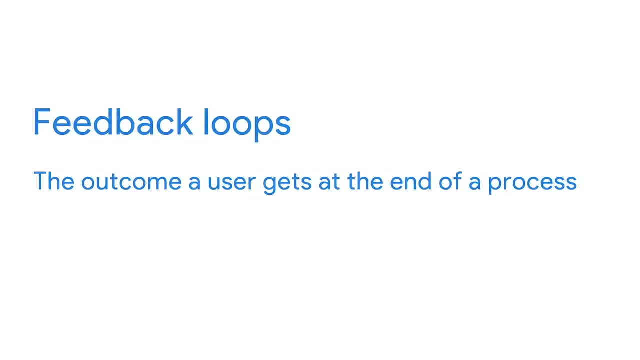 is expected to end with you being able to leave the room. A mental model breaks when you can't go through the open door because, for example, there's a solid brick wall behind it. The next psychological concept is feedback loops. Feedback loops refer to the outcome a user gets at the end. 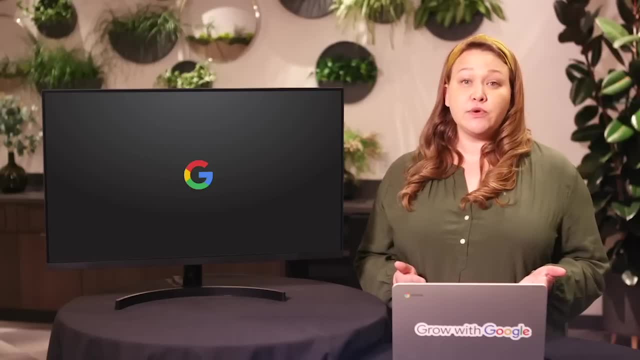 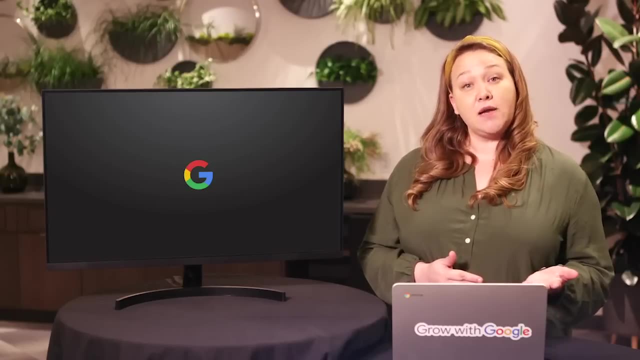 of a process. For example, if you enter a dark room and flip a light switch, the room will either brighten or it won't. Positive feedback would be the light coming on, while negative feedback would be nothing happening. The more positive feedback a user gets when 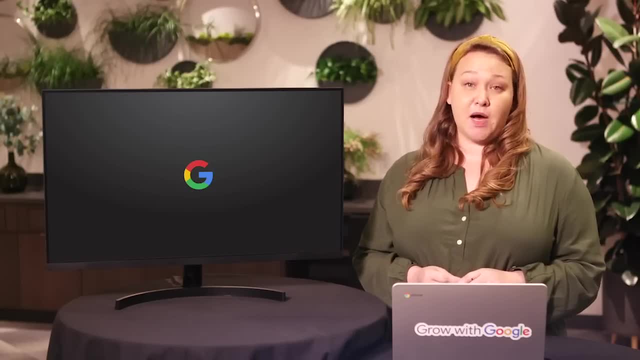 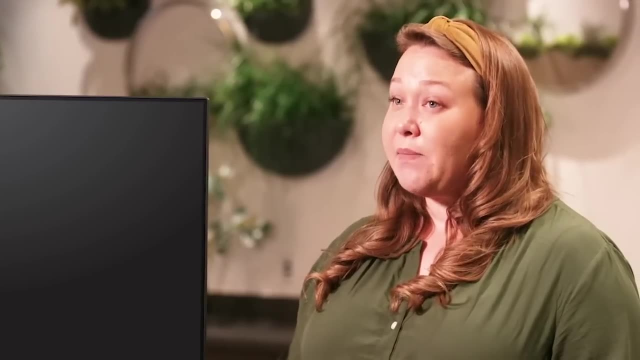 completing the action, the more they will expect the outcome to be positive. The same is true with negative feedback. If your user takes an action, it's important that they get some kind of confirmation that the action worked or that it didn't, In spite of all the limitations, the human 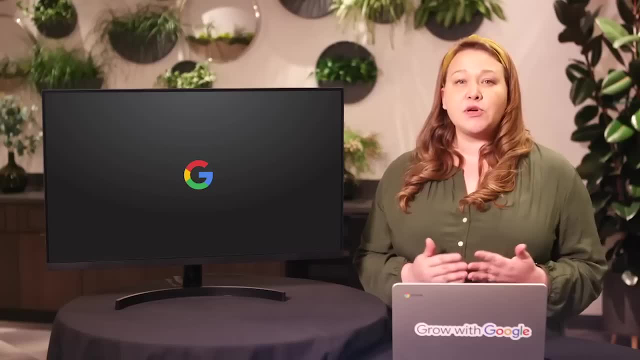 factors puts on the user, the human factor is expected to be positive. The same is true with the decision-making constraints. For example, if your user looks at a small container or says: Here's what I'm doing with the container straw, I'm making it look like it sits on a 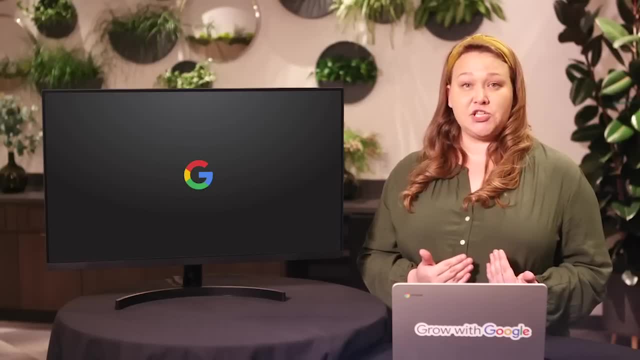 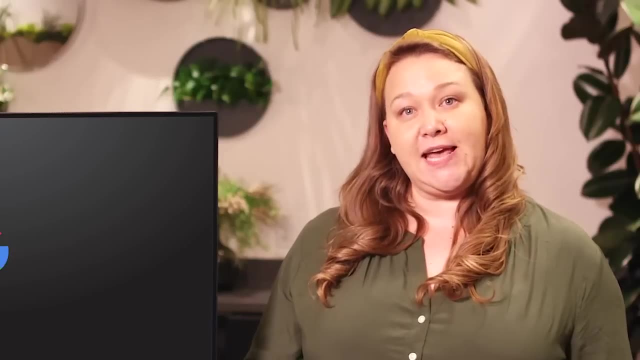 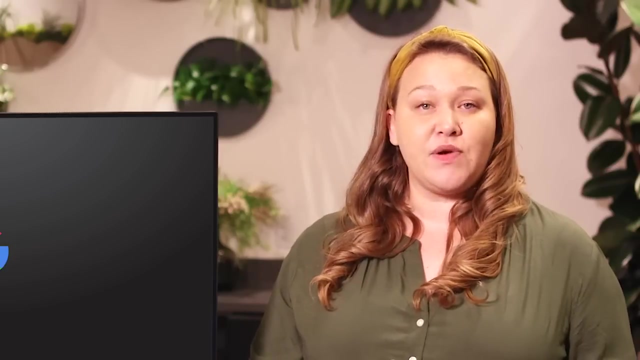 dismissal seat. this gives an action that I immediately М can look at the container and make a suggestion that I normally wouldn't be surprised about. knowledge resources can be used to and can help you get information about stuff you actually want to consider in wished-bad cities Versus with 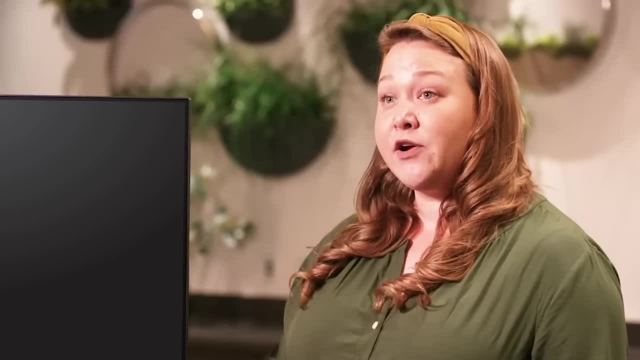 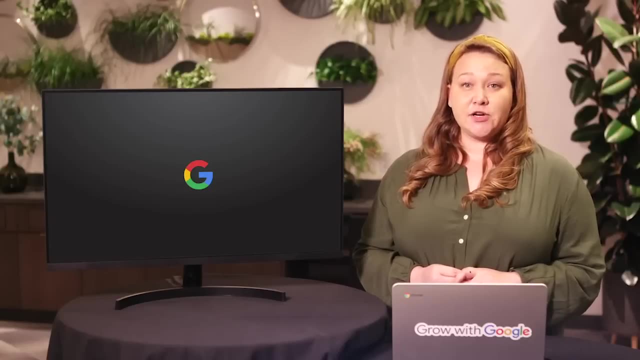 одноatingě. giving your supplier andquently higher vocational skills is marked by the desired. the designer uses nostalgia to connect with users, something they couldn't use to connect with robots. When UX designers turn limitations into opportunities, the human factor isn't so limiting after all. 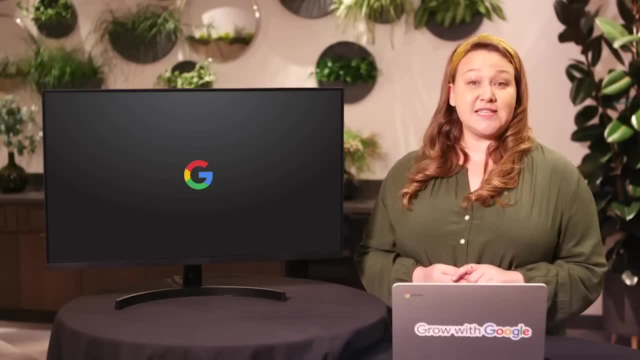 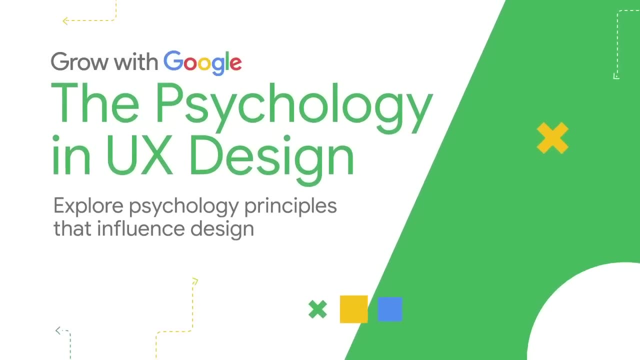 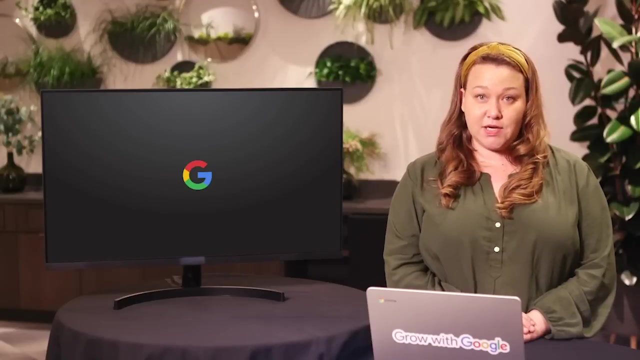 Pretty cool right Coming up. we'll go through some of the psychological principles that act on the user's subconscious as they interact with a product. Sometimes the human factor isn't as simple as lacking concentration or needing motivation. Human beings can be pretty complicated. 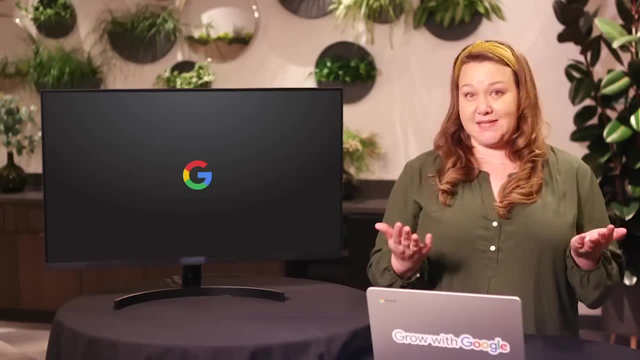 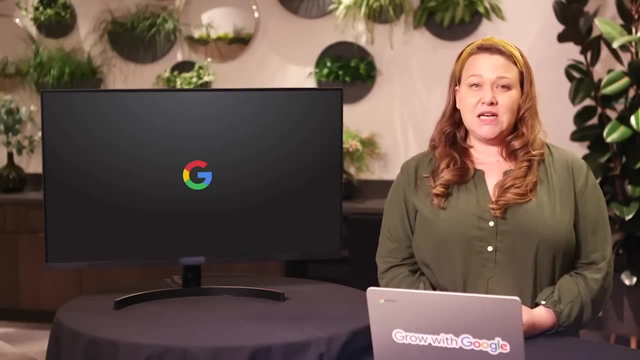 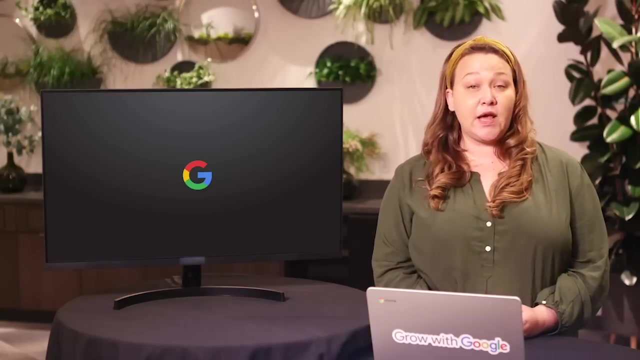 We're always making associations between what we think and what we see. For example, humans usually prefer the color red over the color blue, Why? A 2005 study of the Olympic Games might give us a clue For one-on-one combat-style competitions. 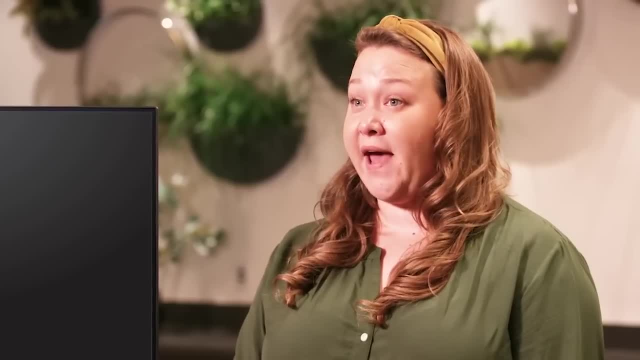 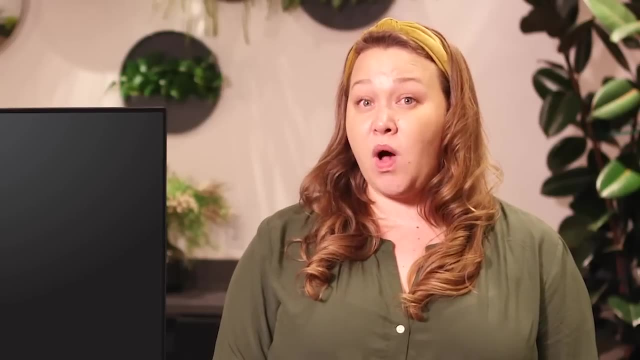 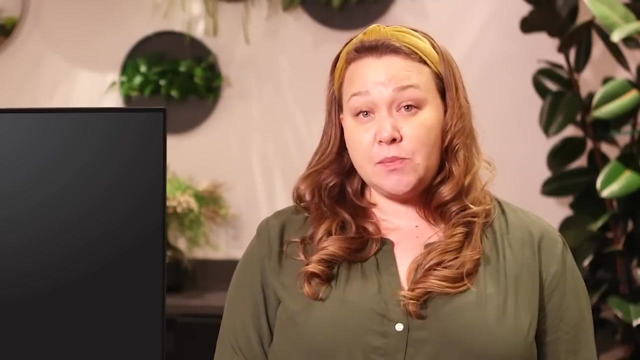 like wrestling or boxing. Olympic rules randomly give one athlete a blue uniform and the other one a red uniform. Researchers discovered that Olympians in red won a statistically higher portion of their matches than those in blue. The study attributed these findings to the human tendency. 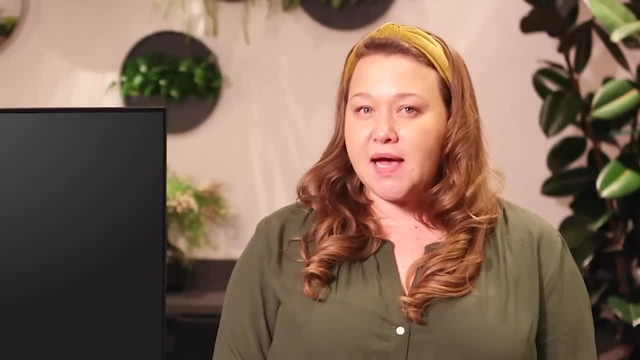 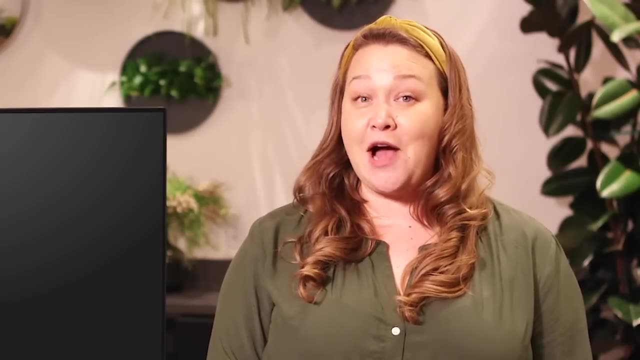 to associate the color red with dominance and aggression. Because of that association, the athletes wearing red were thought to be in a better mindset for a fight. Turns out, the right outfit really can make all the difference. But it's not just color preferences. 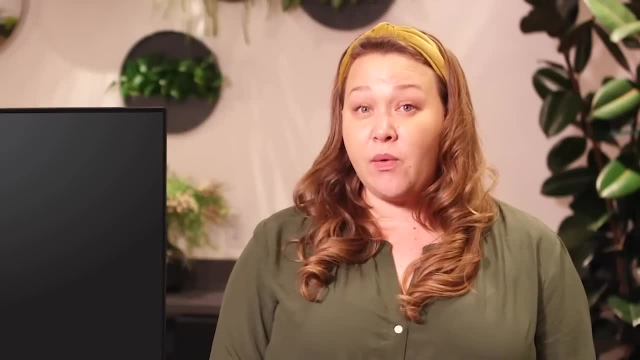 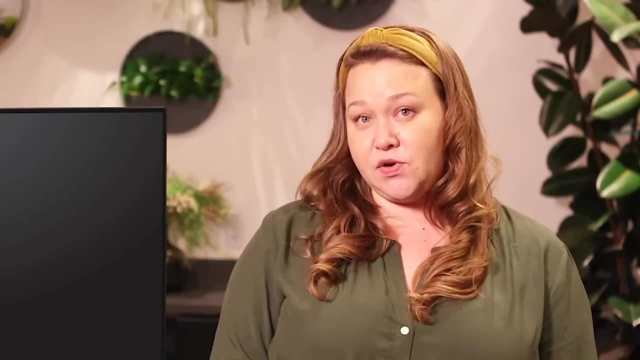 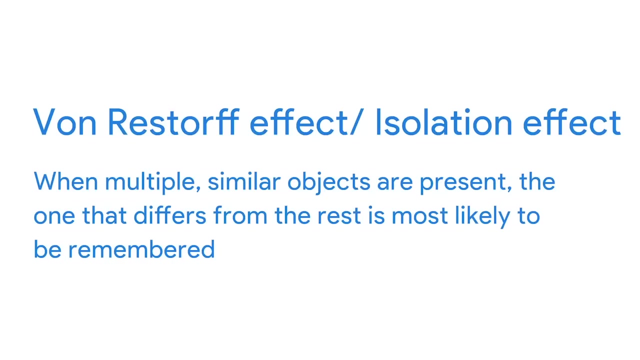 that make humans so complex. Every day, whether we know it or not, we experience examples of psychological phenomena. Let's check out some that can be especially useful to UX designers. The first psychological phenomena von Ressdorf effect, or isolation effect. 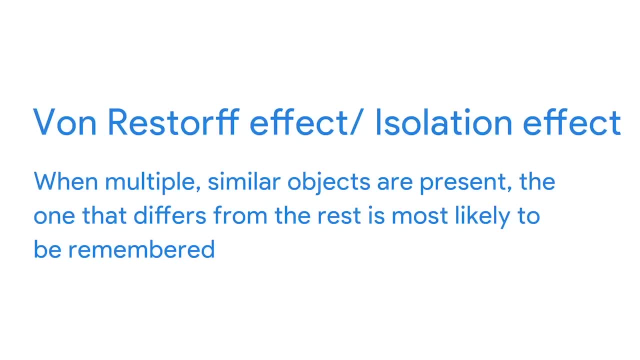 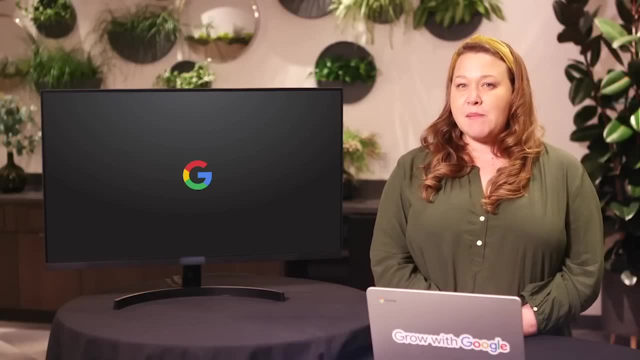 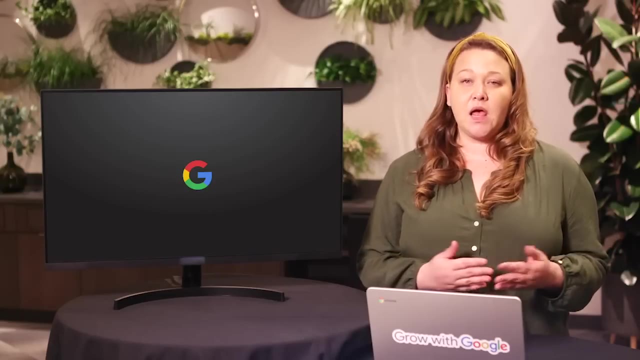 states that when multiple similar objects are present, the one that differs from the rest is most likely to be remembered. Think back to the childhood games you used to play. Remember those spot the difference puzzles. The puzzles were made up of images. Maybe there'd be a picture of three cows. 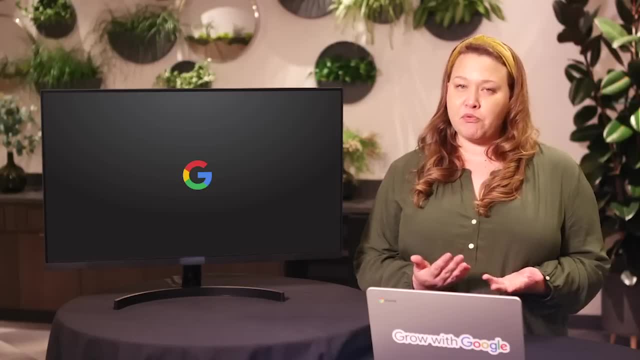 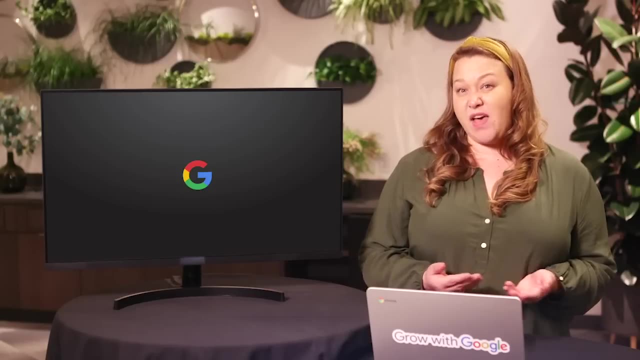 The first two cows are white with black spots and look like pretty generic cows. They fit a young child's definition of what a cow is. But cow number three doesn't have any spots. The von Ressdorf effect tells us that the cow without spots 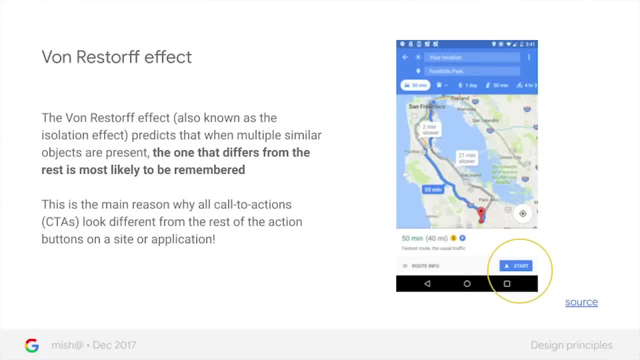 the unique cow will be the one we remember In UX design. this is why the call to action buttons look different from the rest of the buttons on a site or app, Because we want them to stand out. In case you're not familiar, a call to action or CTA. 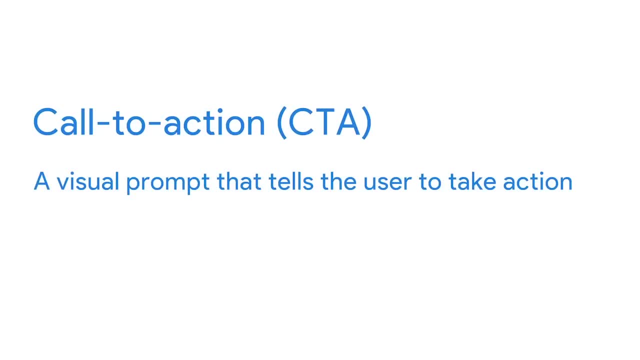 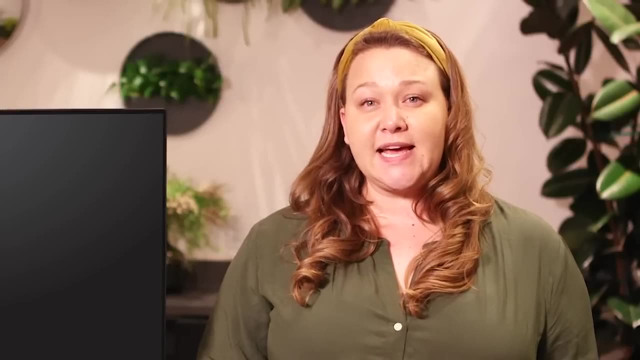 is a visual prompt that tells the user to take action. For example, the start button on Google Maps is bright blue on a white background, which makes it stand out. The second psychological phenomena, serial position effect, says that when people are given a list of items, 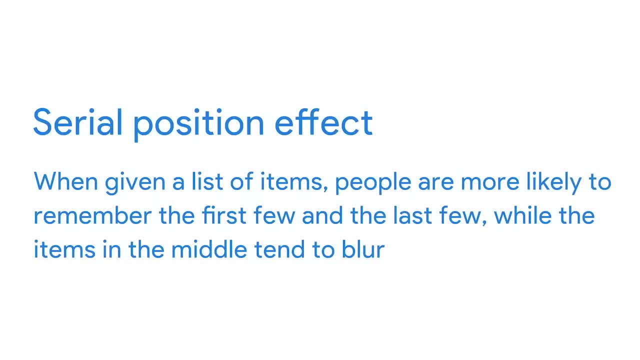 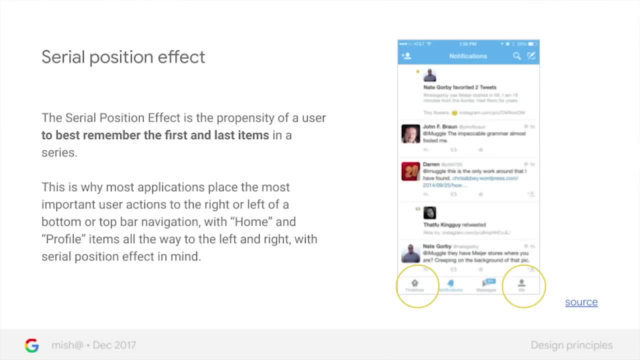 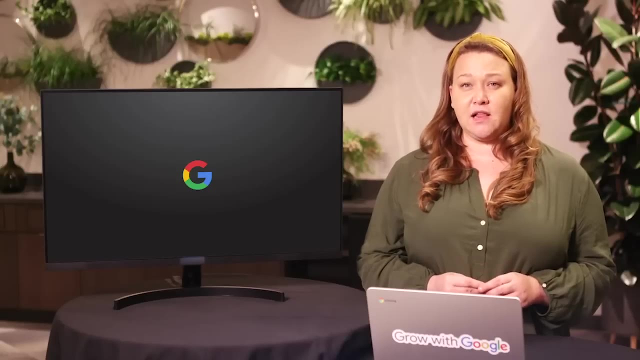 they are more likely to remember the first few and the last few, while the items in the middle tend to blur. This is why most applications and websites position the most important user actions toward the far right or far left of a top navigation bar. The third psychological phenomena: Hick's Law. 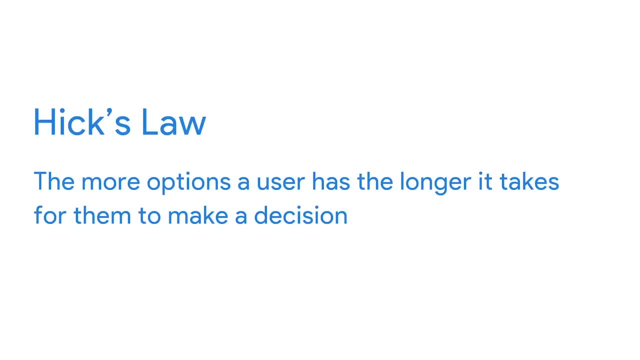 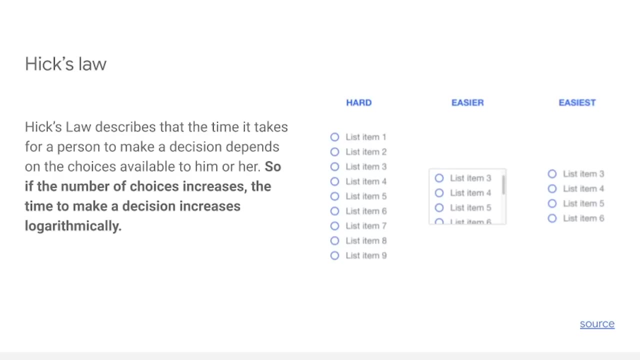 states that the more options a user has, the longer it takes for them to make a decision. We can experience Hick's Law in action in the potato chip aisle of any grocery store. Rows and rows of different potato chips, Even if you narrow your choice to one brand.